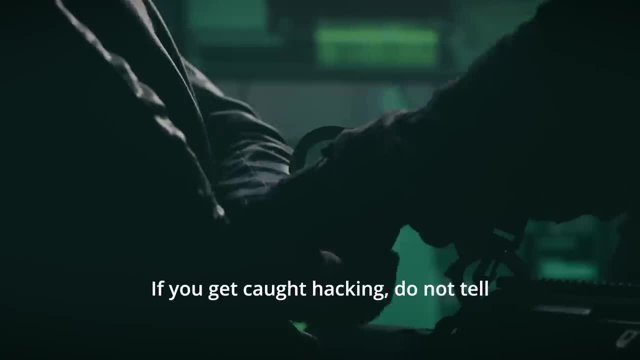 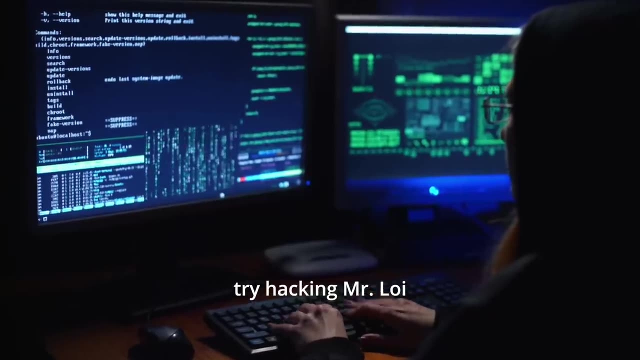 And before we get started, kids remember hacking is illegal. If you get caught hacking, do not tell them. you know who is Mr Hacker Loy And if you want to, you can go ahead and try hacking Mr Loy Liang Yang's website, LoyLiangYangcom. And yes, I promise you I will help you find. 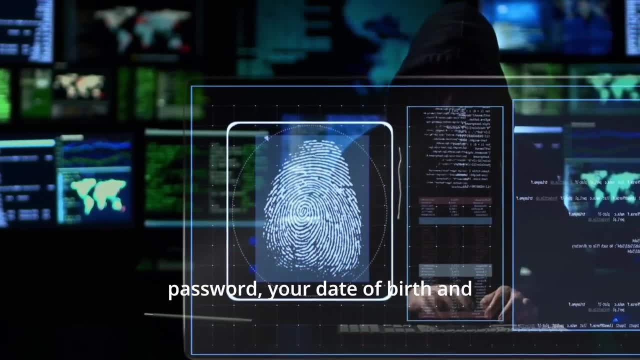 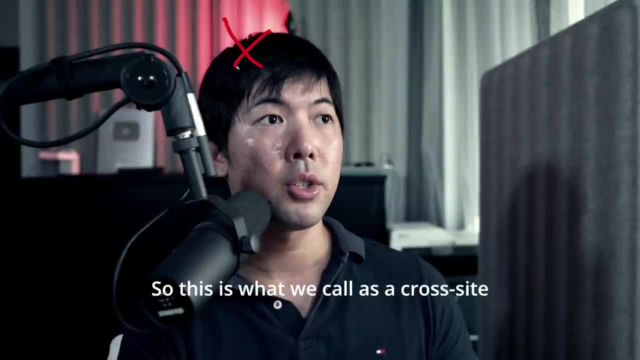 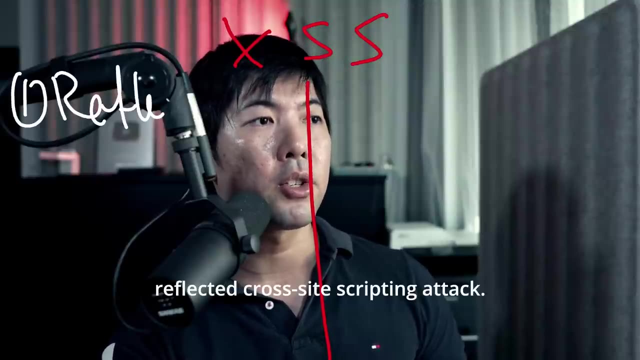 your IP address. I'll help you find your username, your passwords, your data buff and everything about you for free. So go ahead and do that. So this is what we call as a cross-site scripting attack, And there are two forms of it. The first type is what we call as the reflected cross-site. 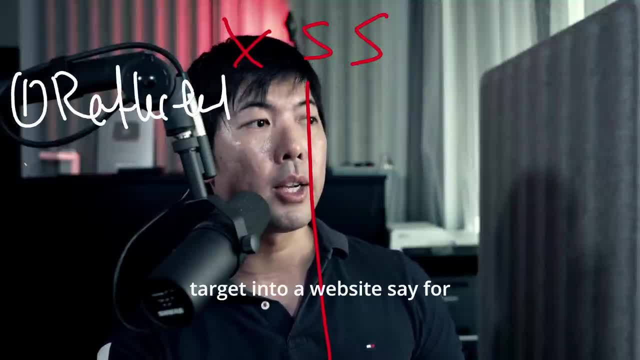 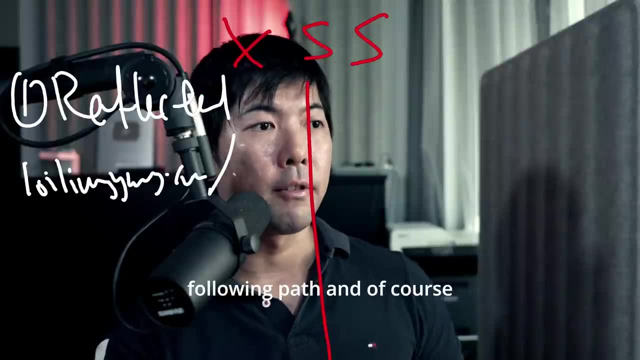 scripting attack, And what it does here is that when you target into a website, say, for example, Loy Liang Yang, What you have here is you have the following path And, of course, in this case you could enter something like JavaScript and you're able to say: capture the cookie information. You're able to. 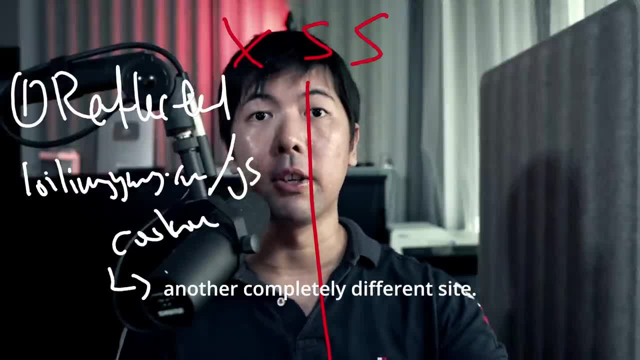 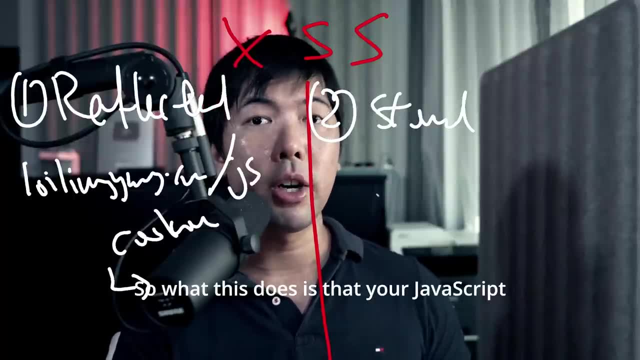 redirect the website into another, completely different site. And the second type of attack is what we call as a stored cross-site scripting attack. So what this does is that your JavaScript, in this case, is going to be stored into the computer back end, usually typically on the. 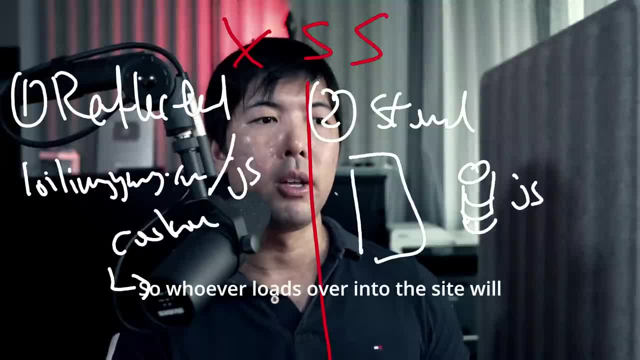 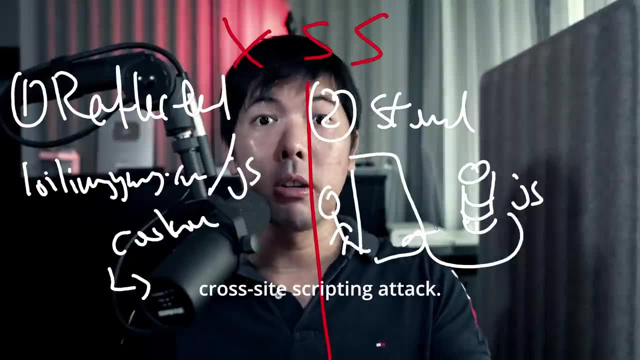 back end database system And you have your code right here. So whoever loads over into the site will load the hacker JavaScript as well. So this is what we call as the stored cross-site scripting attack. And yes, you are correct, We'll be learning both of them. 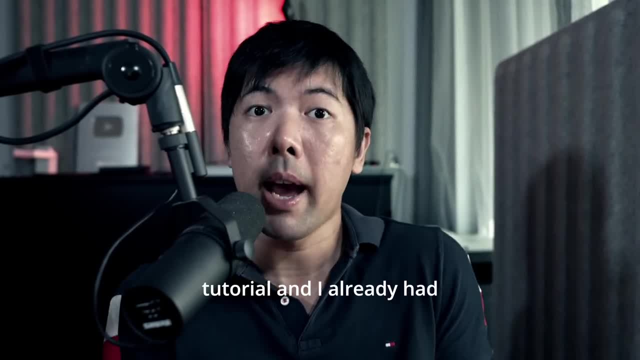 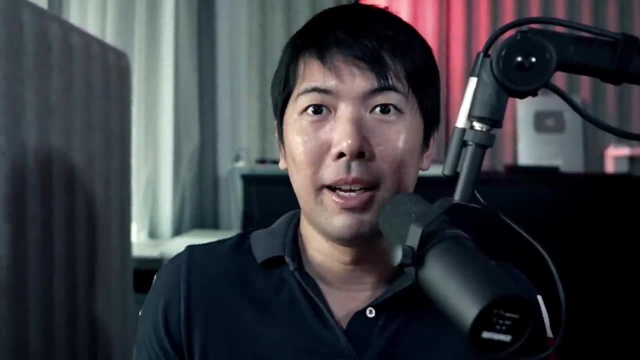 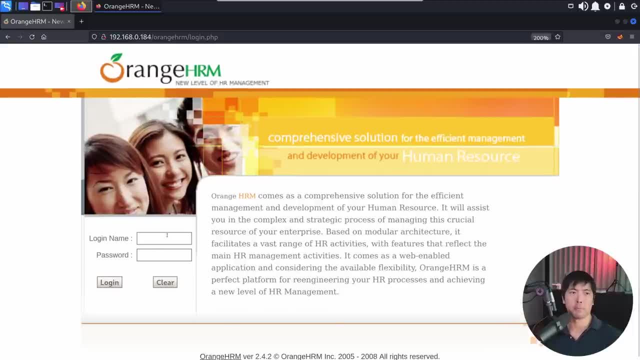 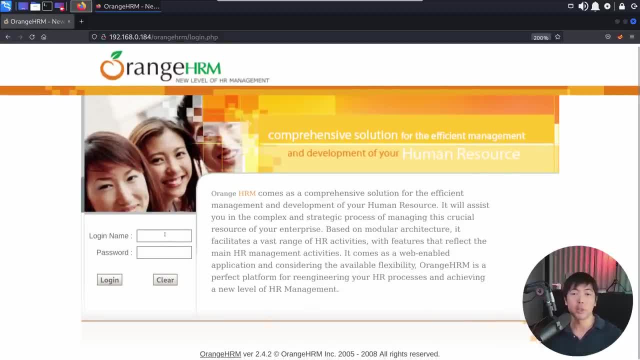 resource management, HR management, And we have a login on the left side, So let's go ahead and enter, say, our login name. All right, So in this case I can enter hackaloy And we have the password of 12345678.. Of course, this is the password to use, especially when you are a popular 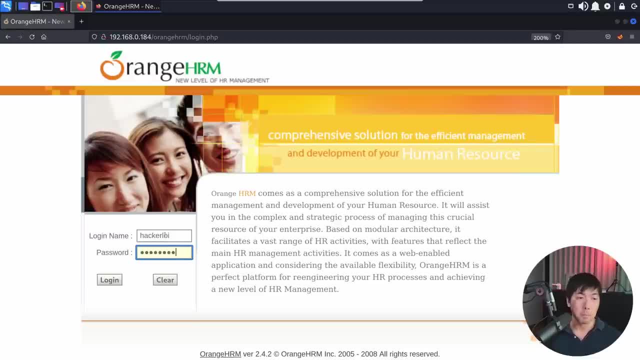 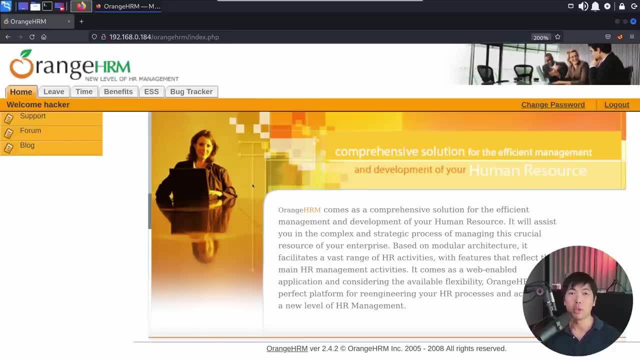 hacker, because people will think that you'll be using a very complicated password. So again, reverse psychology 101.. So go ahead and click on login And right here we're in. All right, orange human resource management system, And what we're trying to do here is uncover the entry. 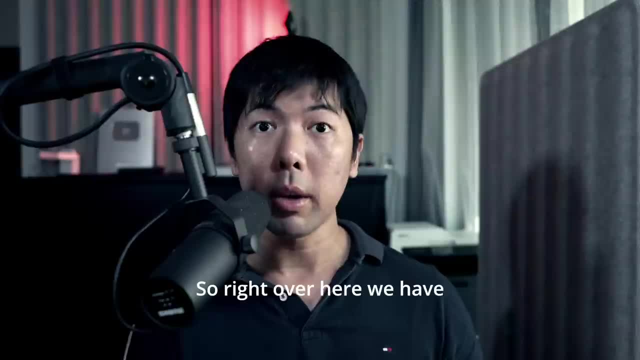 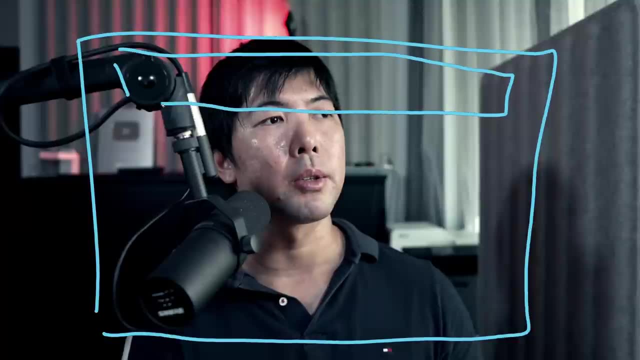 points that will allow us to inject our own script. So right over here we have a typical looking website, And what we're trying to do now is we're targeting the part here which is the URL. So in this case we would have different type of links, pages and so on, And 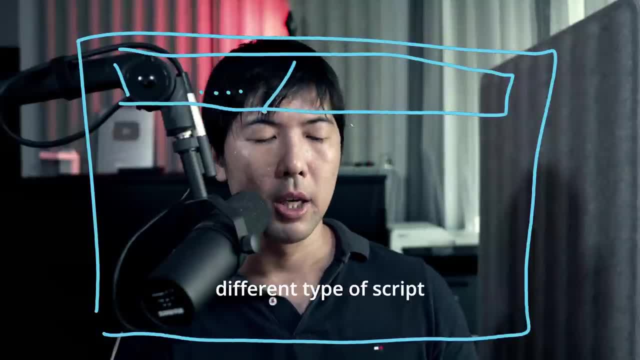 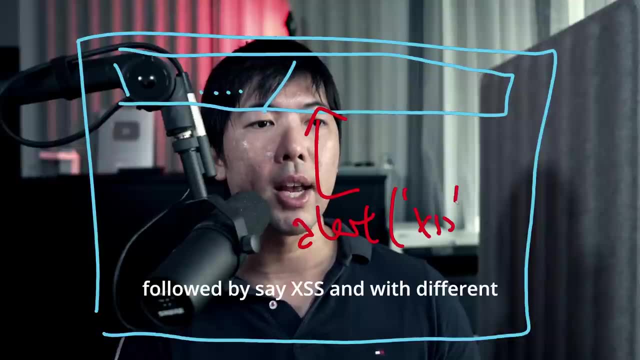 what we're trying to target and attack over here is to inject different type of script into this segment so that we can see whether we're able to do, say, for example, an alert followed by, say, X, S, S and with different payloads, to try it out, And as we inject different type of payloads. 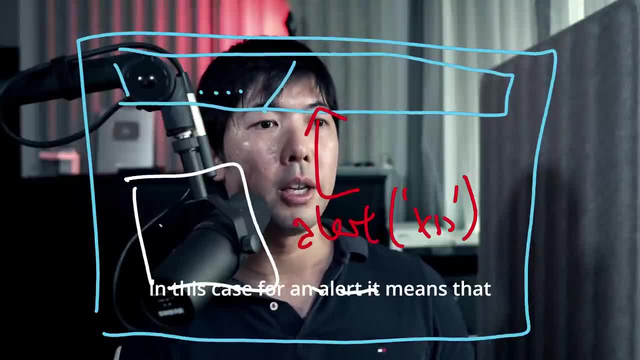 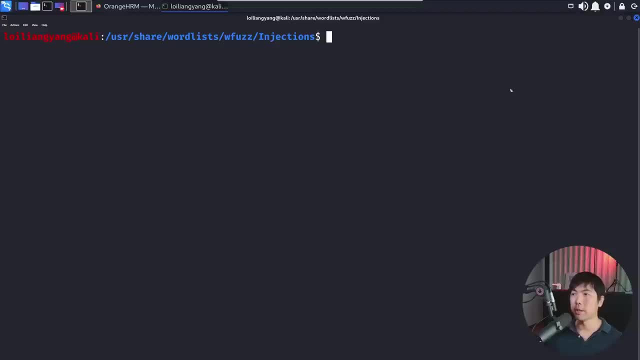 over here and the moment we get a pop-up, say, in this case for an alert, it means that we are able to prove that this segment is vulnerable or susceptible to cross-site scripting attack And you can see over here. we are in the following directory in ColorLinux, which is USR share. 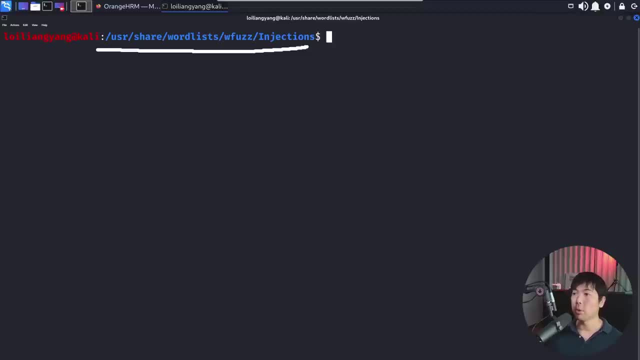 wood list, the BlueFuzz injections, And once we're over here, we're able to go ahead and figure out what are the different type of payloads that we can use as part of again attacking different parts of the URL. So in this case we have XSStxt. So if I go ahead and enter, say, hey, XSStxt, we can see. 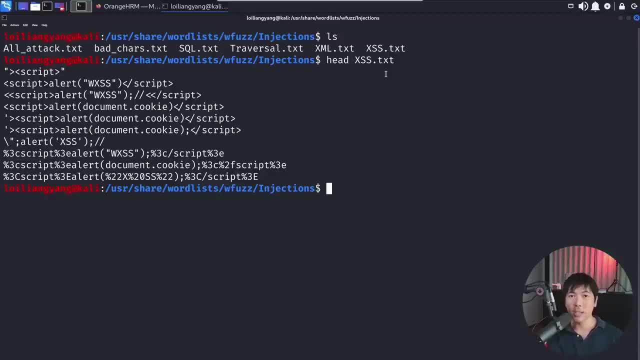 all these different examples of JavaScript that we can inject over into the URL. We can see which one of them is going to allow us to get the pop-up that we want to validate that this segment or this section of the page is vulnerable And, as you can see over here, we have the URL In this case. 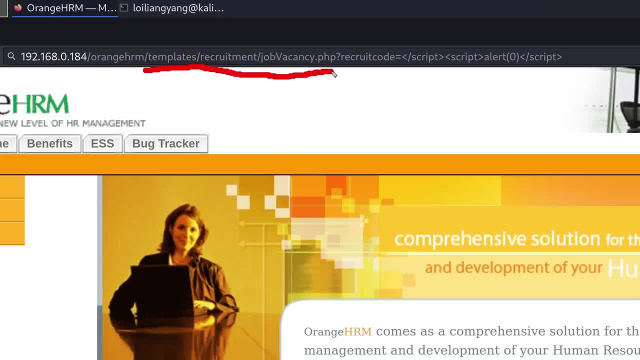 we have going into the directory of templates: recruitment, jobvacancyphp. So this is the target page And we have the following of recruitphp Code: equal. So they're expecting some kind of recruit code And in this case we're ending off. 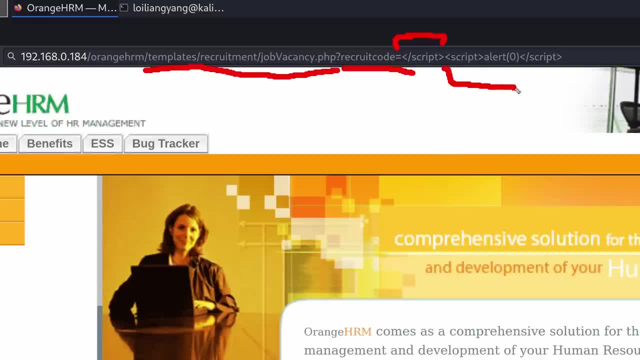 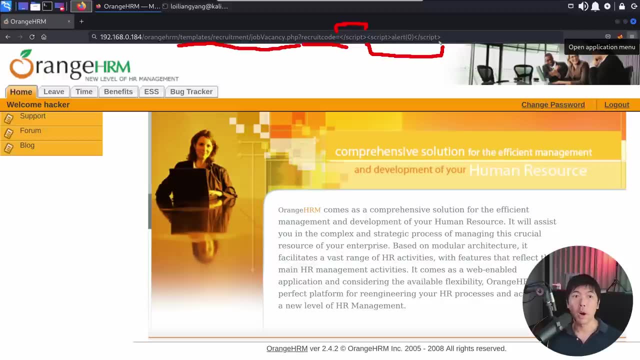 a JavaScript first. So we're ending off the JavaScript and inserting our own JavaScript into the recruit code. So in this case, this allows us to execute whatever script we want to write in here And once you're waiting, in three, two, one, hit enter on that boom. 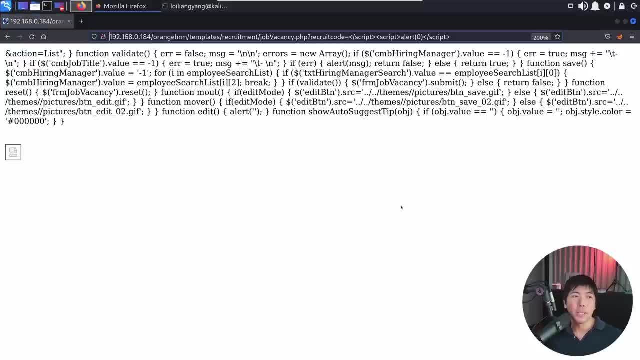 you have this beautiful pop-up, And what does it mean? It means that this part of the page is susceptible, It is vulnerable to cross-site scripting attack. And you'll be saying, okay, so what? What can we do about it? Now, before we go into what we can do about it, 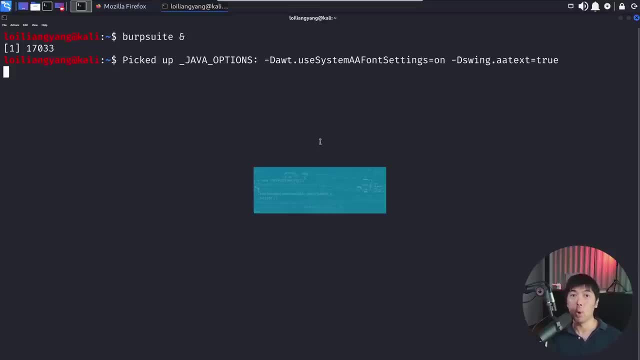 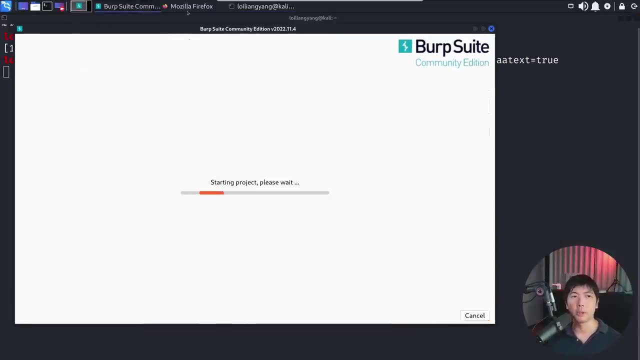 you can also use another tool like Burp Suite to help us load all of those different malicious cross-site scripting payloads over into the target field. So in this case, let's go ahead and start Burp, And what we can do now is go over into the top right corner of the browser. So go ahead and 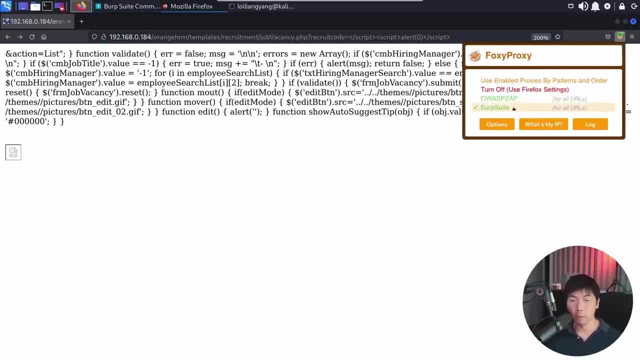 select on it And, of course, use Foxy Proxy. In this case we're targeting over into Burp Suite, So Burp Suite will help us intercept the requests. So once you're in here, all we got to do is. 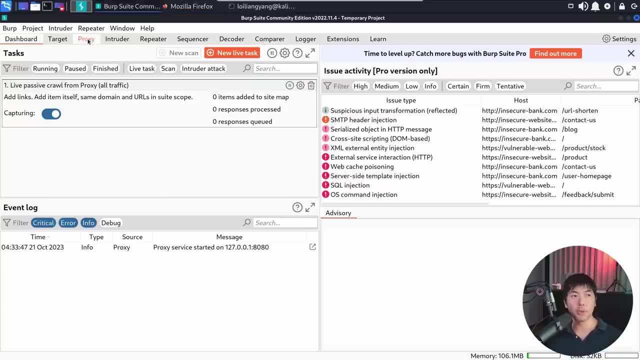 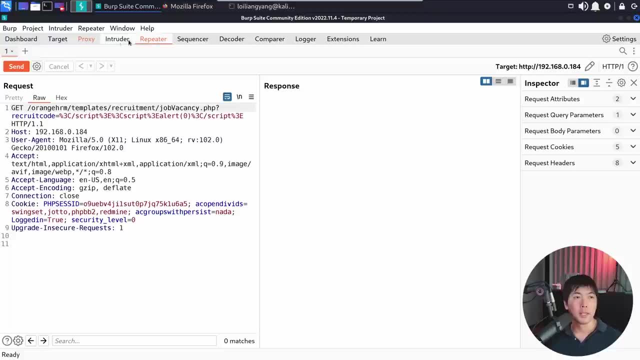 say, for example, I hit enter on this again and Burp Suite under the proxy tab, will pick this up. It will pick this request up And all we got to do is do a right click or send over into- in this case, so let's send over into Intruder. So once you're in Intruder, all you got to do. 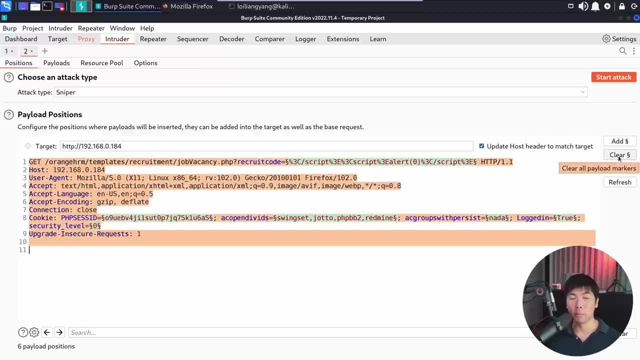 right now is go ahead and clear all those different payload markers And once you're ready, you can just change the recruit code. In this case, maybe I'll put A, And what I can do now is go ahead and highlight this one at the payload marker, go over on the payloads. 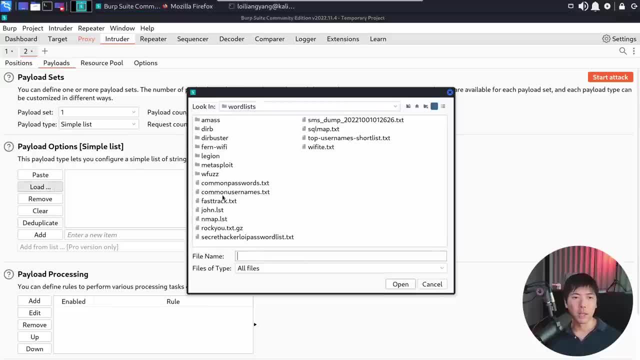 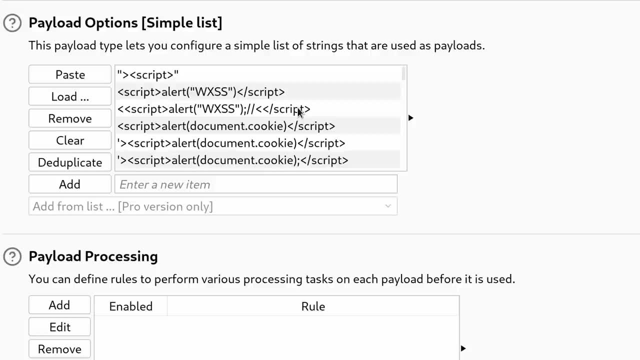 click on the load. So in this case we're wordless And of course we can go over in the directory that we were at earlier under WFuzz, under Injections, under XSS. So here we have all this different cross-site scripting attack payloads that we can use and start. 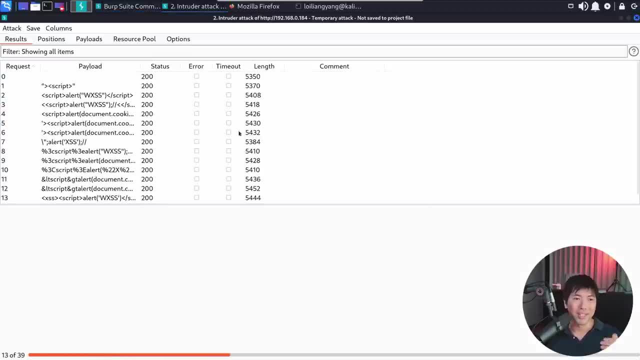 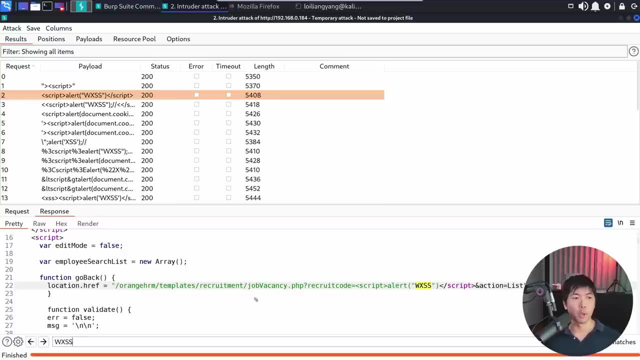 attacking, hammering away into that specific view, right, And we can see the length and see what is the potential response to it. So if you would investigate a little deeper, you can see right here we have the following: The function go back right. So in this case, 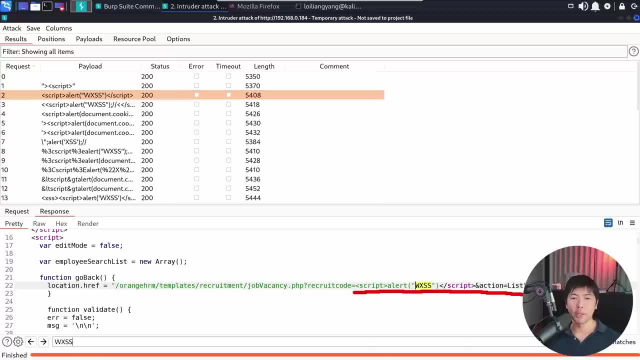 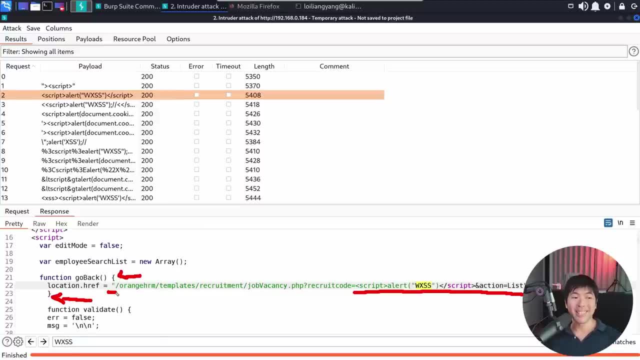 curly braces, all right, as well as another curly braces over here. So if we can escape away from this following, it means that this will allow us to run our own JavaScript onto the site. So this is genius. So, extracting that piece of code over here, you can see the following: 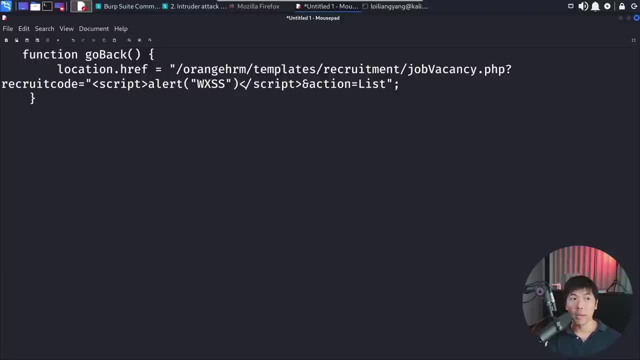 If we could terminate from this end with a double code and then followed by say a curly braces to end it all off, And then from there on we're. then you can see that the payload has been supplied over here And you can see the function has the. 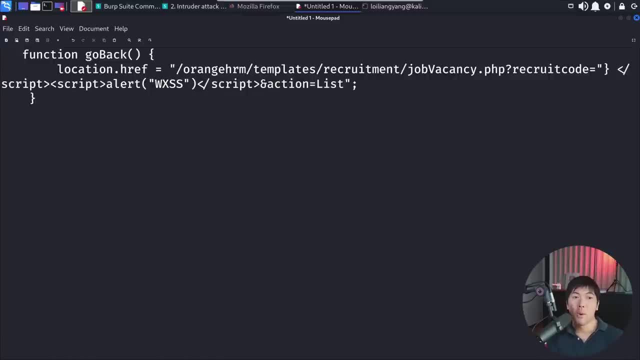 curly braces to end it all off. And then from there on we're, then you can see that the payload has been supplied over here, And then from there on we're able to say close off possibly the script and then inject our own script into it. 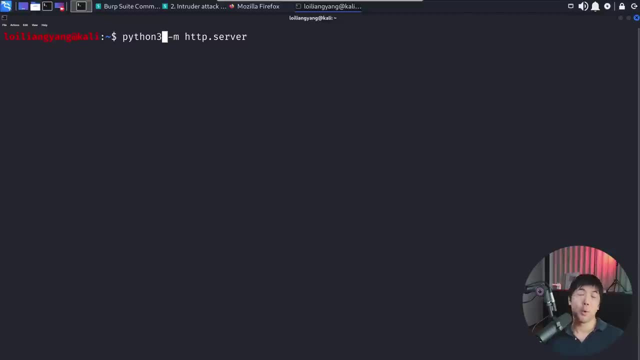 which is why the initial payload that you saw earlier was working. So what we're going to do now is we don't know the username or the password, But what we could possibly do is sort of hijack their session. So what I can do now is go ahead and use python3-mhttpserver And we're starting. 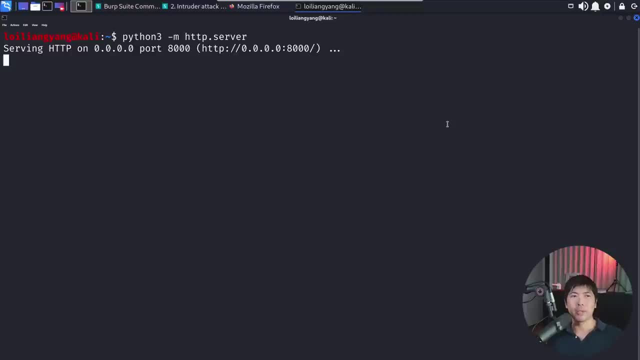 up our server So anytime we can redirect all those session information from the user to the hacker. So in this case, what I can do now is go ahead and craft out a more specific payload that allow us to do just that. So you can see, over here we have the documentlocation And we're 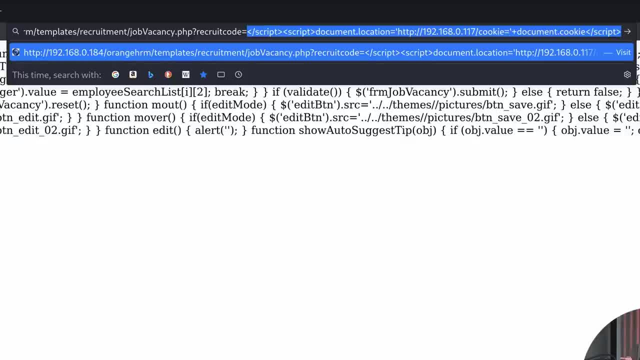 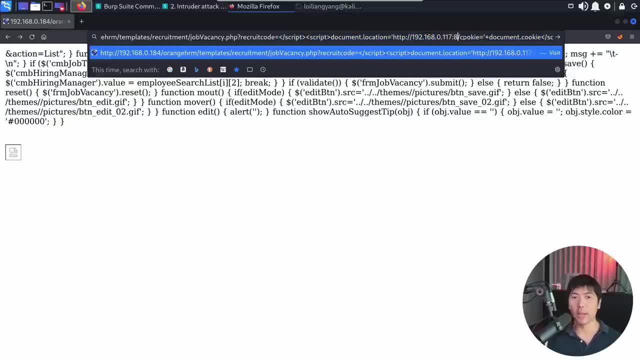 forwarding this over into the hacker's IP address, right? So in this case, let me just go ahead and double check on this. This is on port 8000.. All right, so let's go ahead and fix this up a little bit. So let's go ahead and enter port 8000 for this And, once we're ready, in three, two, one. 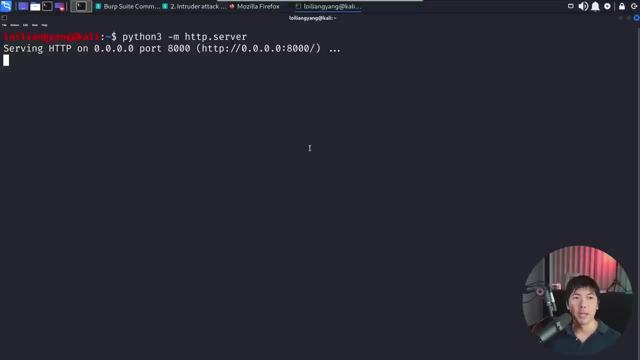 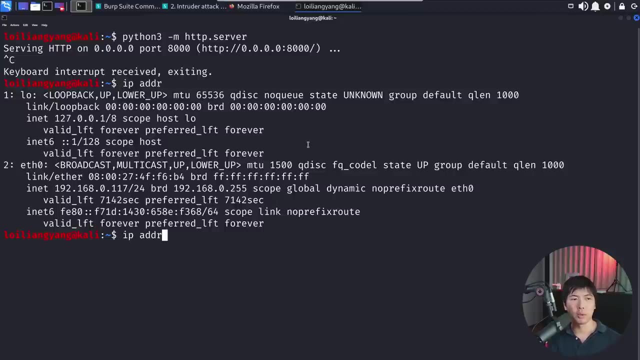 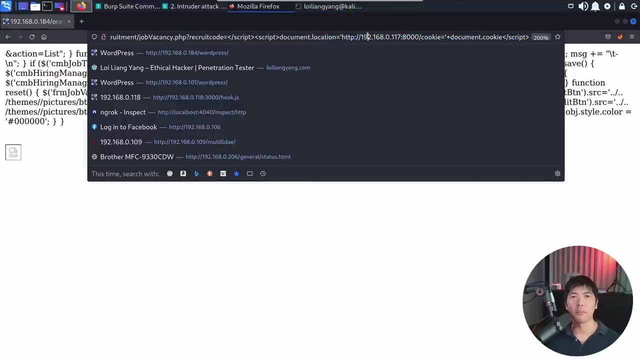 hit enter on that. Go back over into terminal and see what we get. All right, nothing for now. Let's go ahead and start it up again. Hit back over into the payload, All right. so in this case we have documentlocation. We have the following of documentlocation: 192.168.0.117, port 8000. 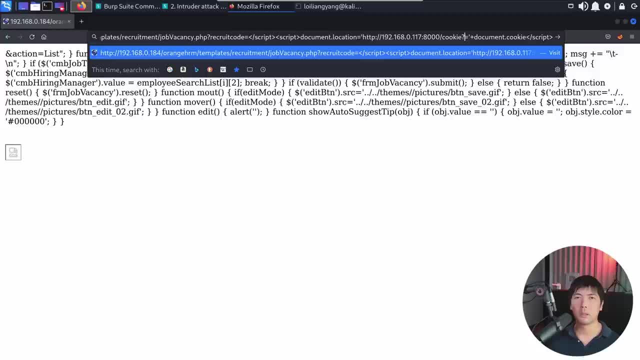 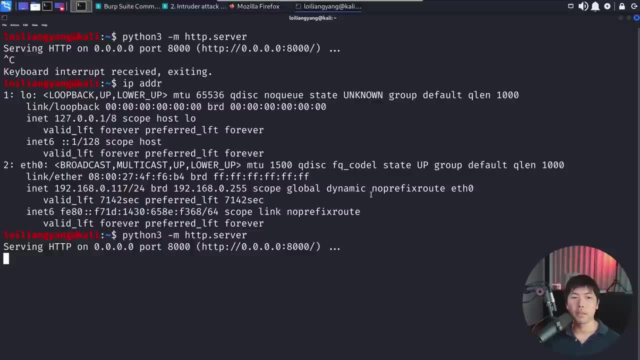 slash cookie equal. Okay, let's go ahead and troubleshoot this one. Okay, I've added a question mark over here, So let's go ahead and hit enter on that And let's see what we get this time around. All right, still nothing, but no worries, Let's go ahead and try something else. 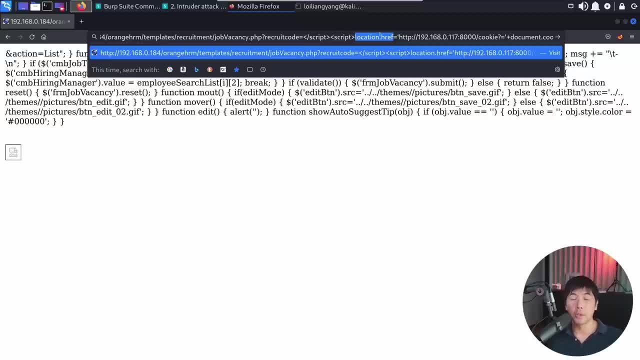 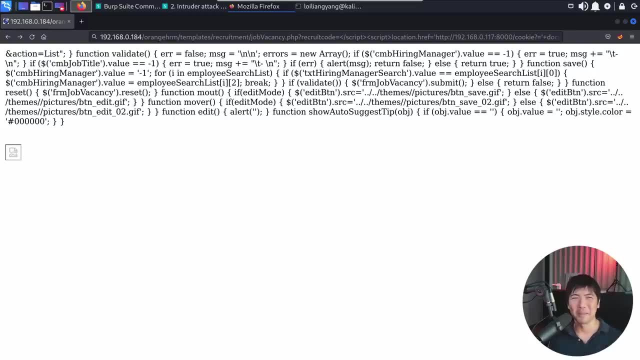 Now what I've done here is I've changed this up to locationhref. So let's go ahead and hit enter on that, Go back over to terminal, Let's see what we get. So you know what's the problem. The problem is because there's numerous special characters in 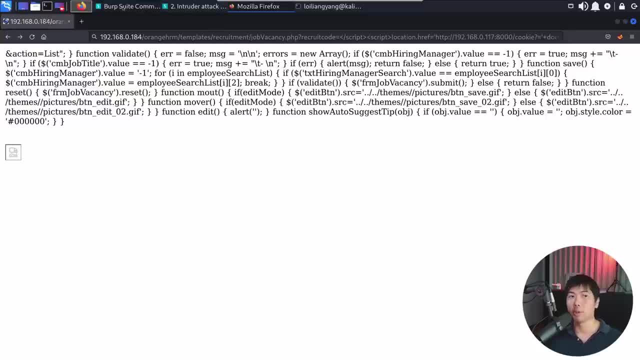 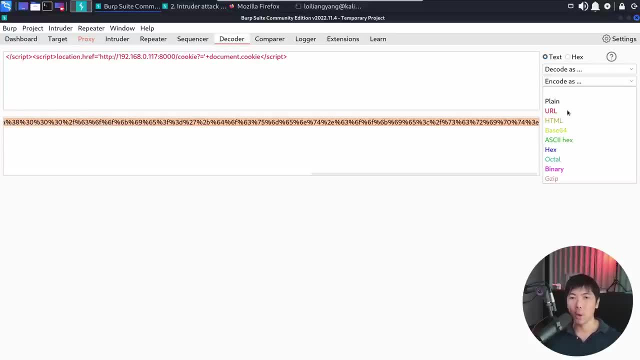 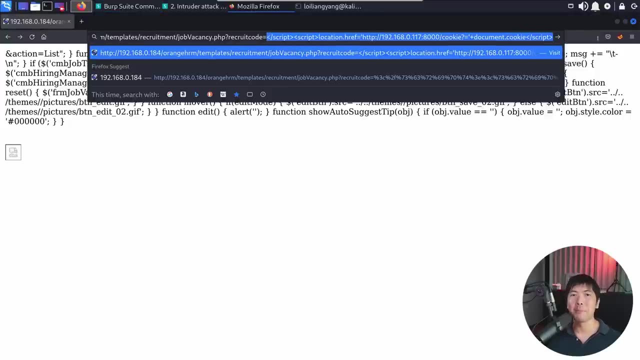 here And what we need to do then is to encode it So we can go back over into BurpSuite, go to the decoder tab, copy and paste the payload over here and go to the right side and select as encode, as URL. So once we have this, we can copy, go over into the browser and replace this. 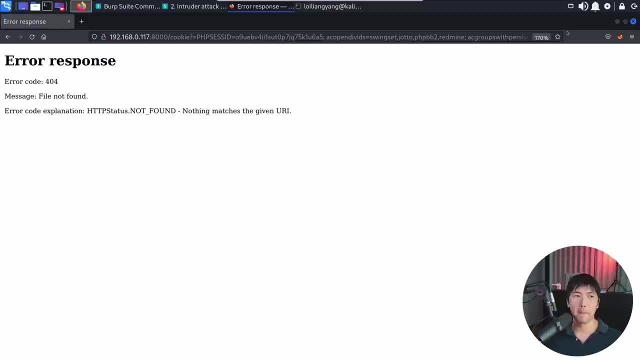 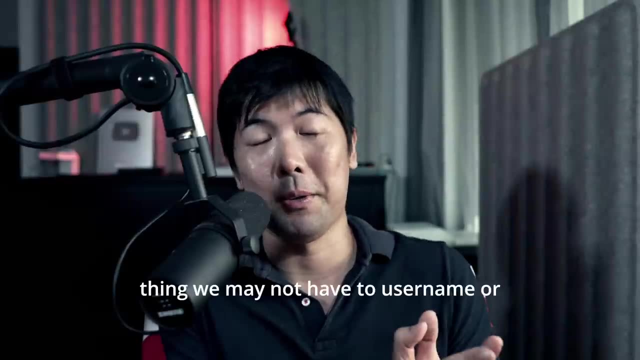 one. Once you're ready, in three, two, one, hit, enter. Now go back over to terminal and see what we get. Boom, you're in. It's game over. So here's the thing: We may not have the username or the. 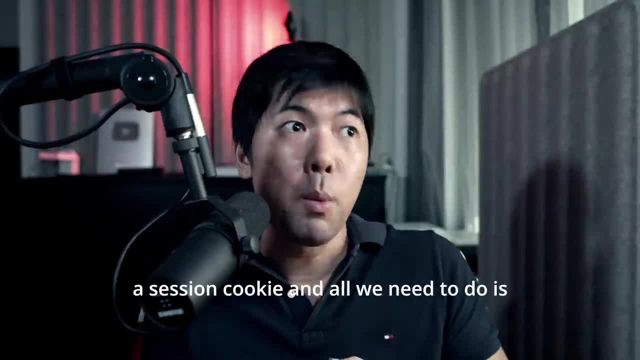 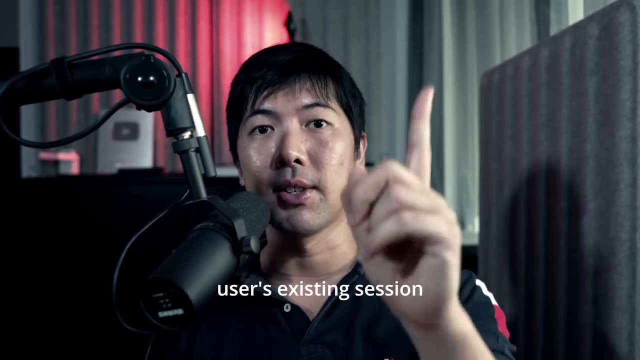 password. It doesn't matter. What we have here now is a session cookie, And all we need to do is to copy and paste those information over into our browser, And that's it. We would gain access to the user's existing session. Now here I am in a completely different browser. I go to the top. 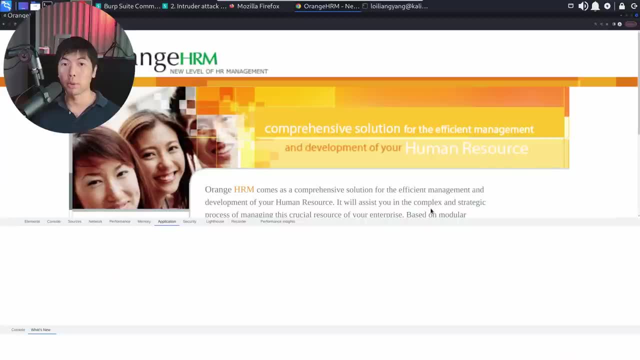 right corner and I select under more tools, And I go to the top right corner and I select under more tools, And I go to the top right corner and I select under more tools, And I go to the top right corner and I select under developer tools. So once I'm in here, what I can do now is go ahead. 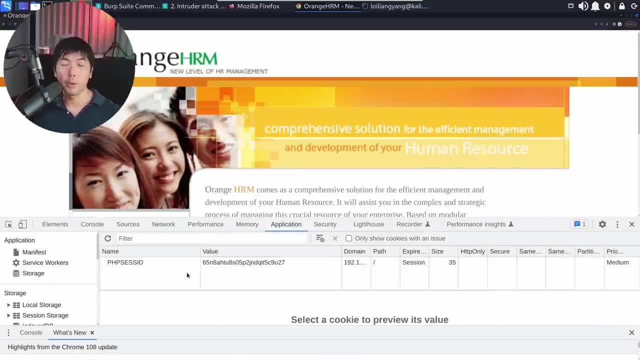 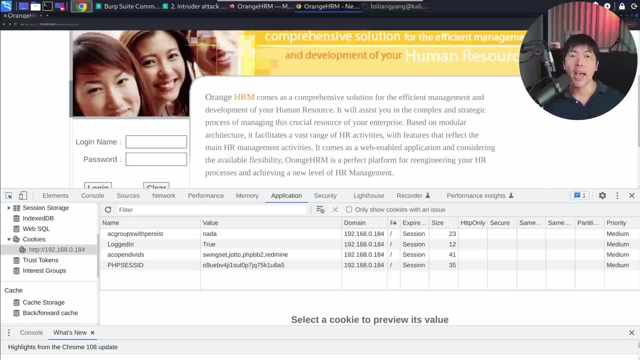 and enter those different name as well as the value that's been assigned for this particular site. All right, So now we've got all the values, all the cookies, right here. This is the hacked values And you can see over here we have not yet went over into one part of the site, which is the. 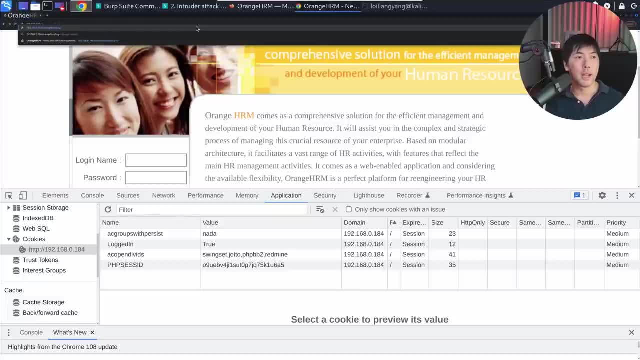 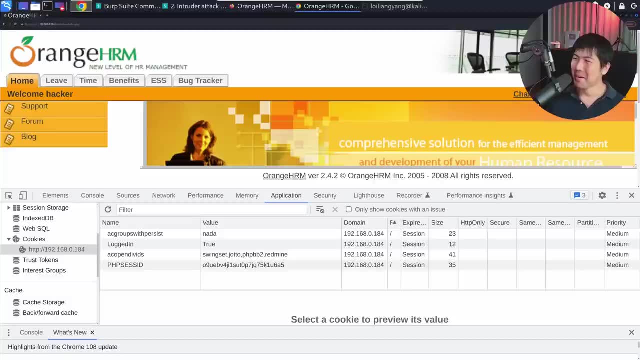 indexphp. So once we're ready, all we can do now is go over into URL and enter the following of indexphp And once you're ready, go ahead and hit enter on that. Boom, We are in. I can see right here. welcome hacker. So now we have gained access to the user session. 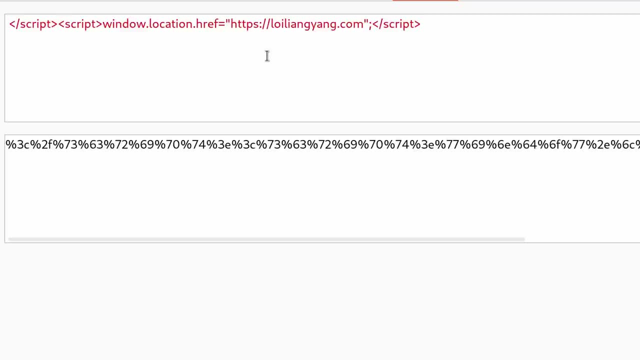 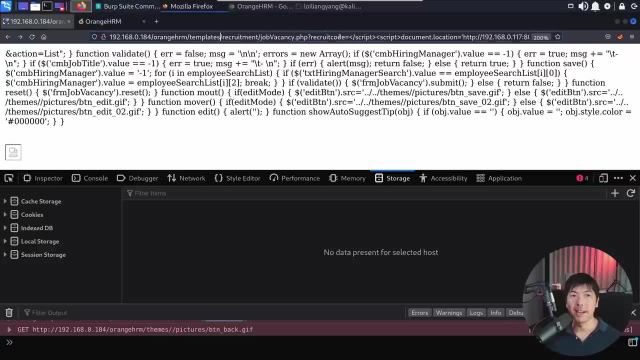 The other payload that we have here is to redirect the user into lloydliangyoungcom. So this is super neat. So if I go over into the encoded payload, I go back over into the browser and replace this payload over here with the encoded payload. I hit enter on that. Watch this carefully. 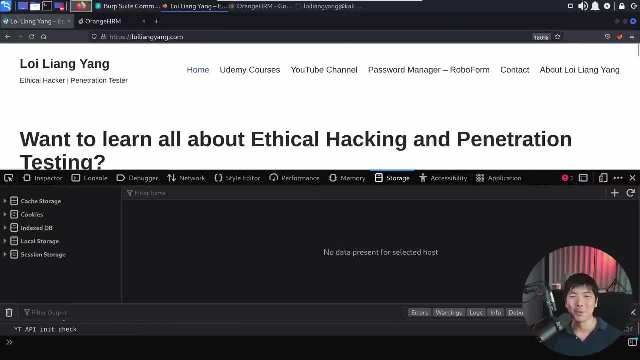 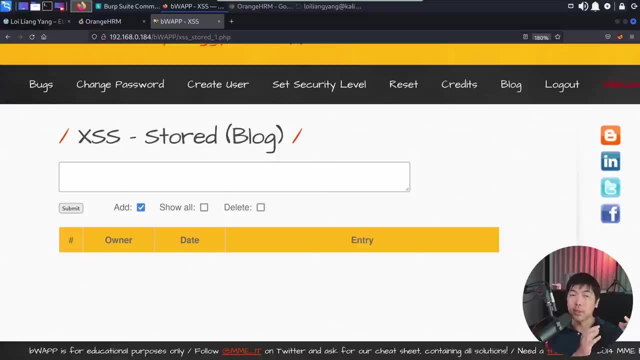 Hit enter on that Boom, We are now brought over into Mr Hacker Loy's website. Now, moving forward, we're going over to the other type of cross-site scripting attack. So in this case it's a stored cross-site scripting attack. What it does is that our code, our script, will now be stored into a